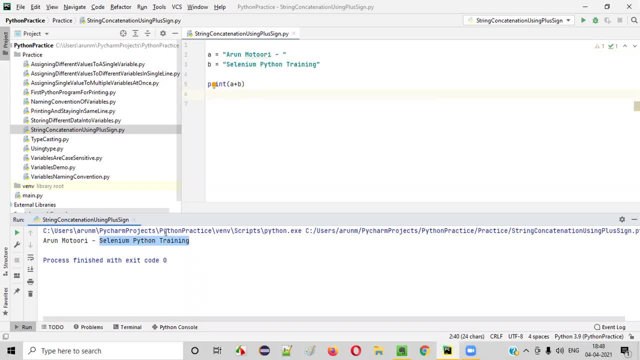 Space got clubbed with the second string text. That is nothing but concatenation. guys, String concatenation. Selenium Python training got printed here. Fine, So far, so good. Now what I will do is, instead of printing A plus B directly, what I will do is I will create another variable. guys Say C is equal to. I'll say A plus B. Here also, same thing will happen. 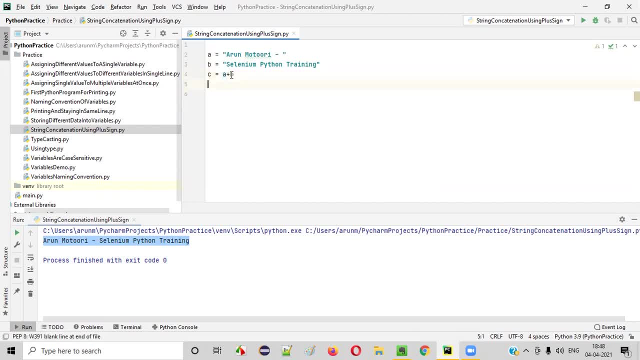 In the variable A we have Arun Moturi space, hyphen space. In the variable B, we have Selenium Python training. These two string texts will be concatenated and the result: Okay, The combined string text, that is concatenated string text, will be assigned to the variable C. Now, if you print C, what will be printed? 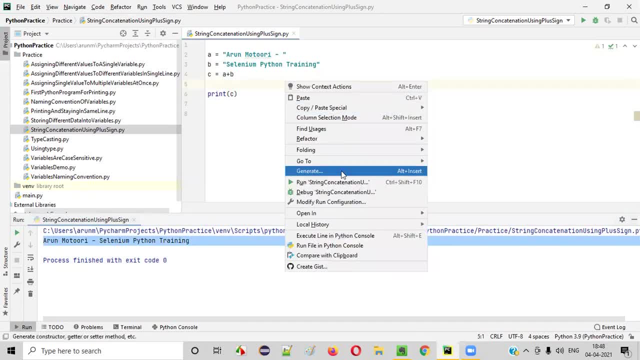 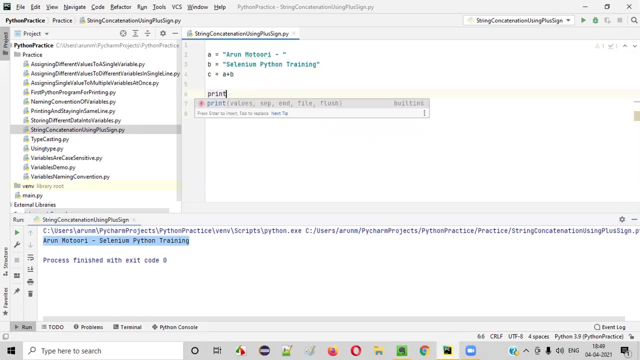 The same result will be printed. guys, Okay, Concatenated string text will be printed. here. You see, Arun Moturi, the two string texts got printed as a concatenated string text. Fine, guys. So that's what. Now we can use something, guys, Okay, We can do one thing. So here I'll say: print. If I print A, what will happen? 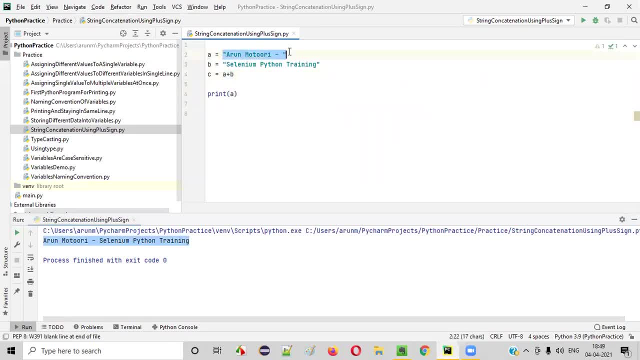 Okay, If I print A, what will happen? Only Arun Moturi space, hyphen space will be printed. Right, Right, Vikran. Only this got printed. Now, if I write some double quotes, Okay, Before this particular variable, if I write these double quotes and I'll provide some string text here, guys, Okay, 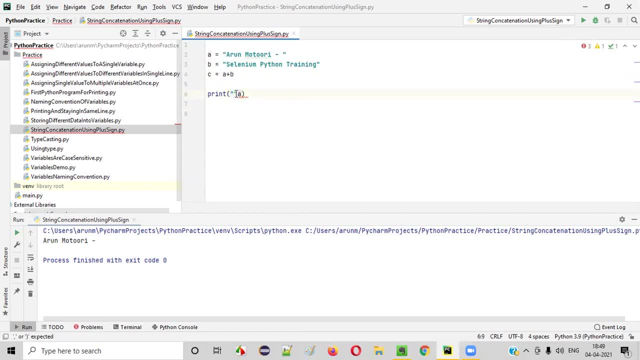 In the print statement. I'm directly hard coding the string text. Okay, Here I'm saying: my name is Okay, My name is From here to here. Okay, Whatever I have written inside the double quotes is nothing but a string text. 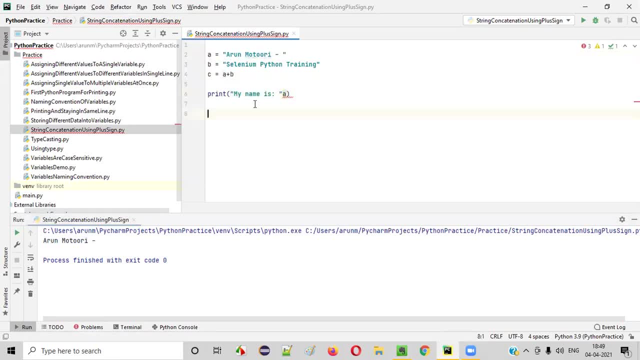 Here, A is also a string text. Right, A is also a string text, and also this is a string text. You are already getting an error, guys. Okay, And the reason here is you have to use the plus sign here for concatenation. 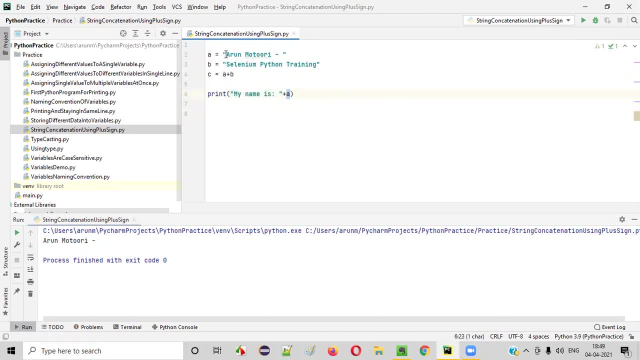 Okay, We have this string text. If you have to concatenate with another string text, that is, Arun Moturi here, which is stored in the variable A, we have to add the plus sign. You are concatenating this particular string text with the variable A. So what will be the result? guys, My name is. 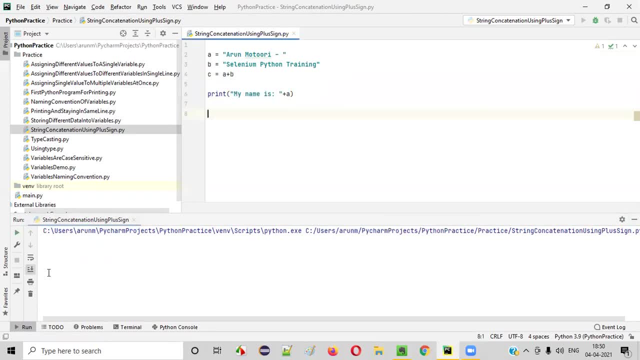 Arun Moturi and the remaining stuff will be printed here. You see, Rightly run, My name is Okay. This particular string text that is my name, is got concatenated with the string text that is stored in the variable A, That is, Arun Moturi and other stuff, and printed like this: 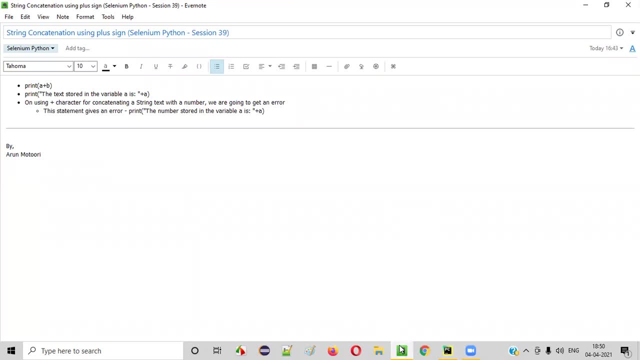 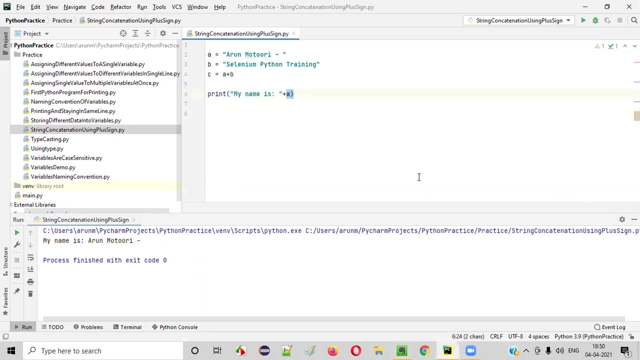 Fine, So this is another way, guys, This is another way. So there is one more thing we have to understand, guys. Here we are concatenating the string text with the variable. Okay, Here we are concatenating the String text with the variable, which is storing the string text itself. 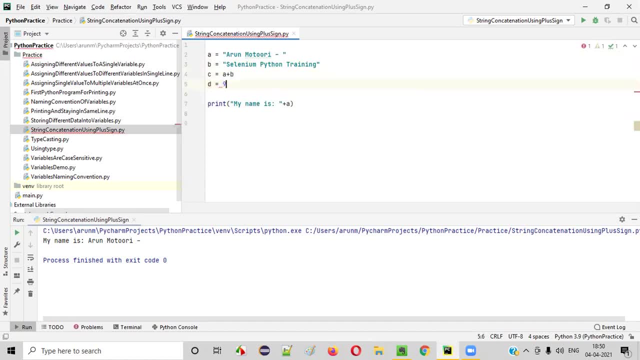 I'll do one more thing here. I'll create another variable, say D and say nine. Okay, Here the variable D is assigned with some integer value, not the string text. What if I change this A to D? It will work. 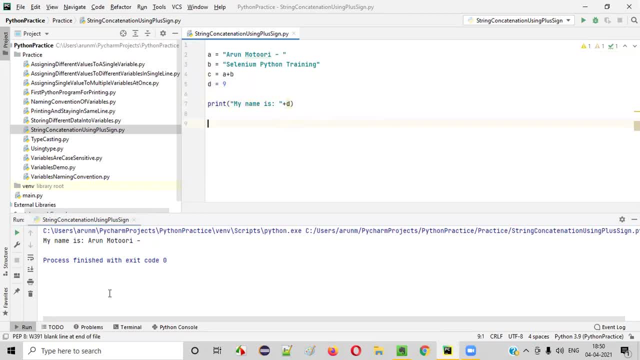 Here. it will not give error, guys, but when you run this code, you will get an error in the output. The reason here is this plus sign in Python. Okay, This plus sign in Python Will only concatenate the string text with another string text. 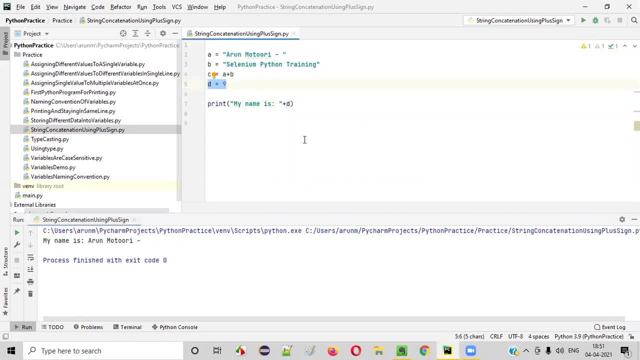 But here, D is not a string text, guys, D is an integer value. So what will happen when you use the plus sign for concatenating the string text with a integer value? You'll not get the proper output. You'll get an error, guys. Okay, I'll show you. you'll get some kind of error. Let me show you Rightly run. 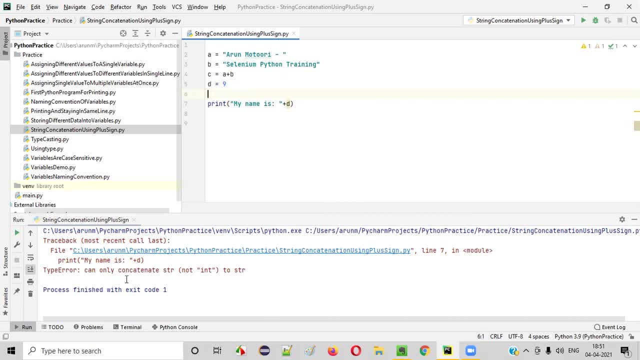 You'll get this kind of error saying Can only concatenate string with another string, but here you're concatenating the string with what You're trying to concatenate the my name is string with the integer Okay, Integer value, which is stored in the variable D. 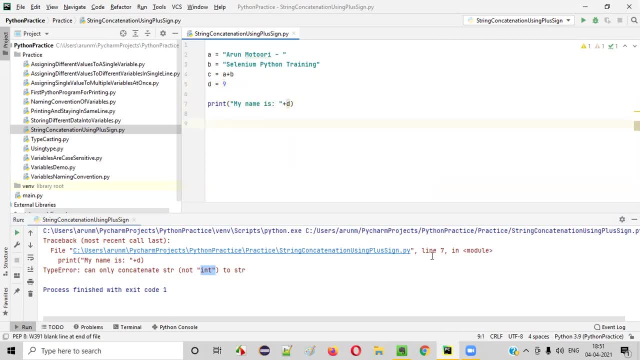 That is a problem, guys. So in which line we got this? uh, issue line seven. Okay, Line seven: this print statement which is trying to concatenate the string text with the integer value. So here, if I say E is equal to A plus E is equal to A plus D. if I say: 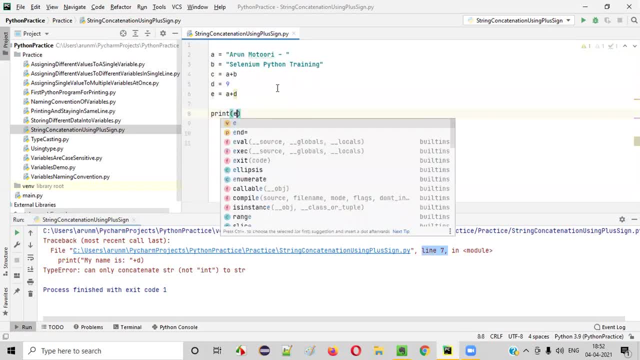 And if I try to print E, same result you will get. If I try to print E, same result you will get. Because into the variable E you are assigning the result of string text getting concatenated with integer value. Is that possible in Python to concatenate some string text with the integer value? Here, Arun Moteri is getting concatenated with the integer value nine. That is not possible, guys. If you're trying to print E, you'll get the same error again. Rightly run.